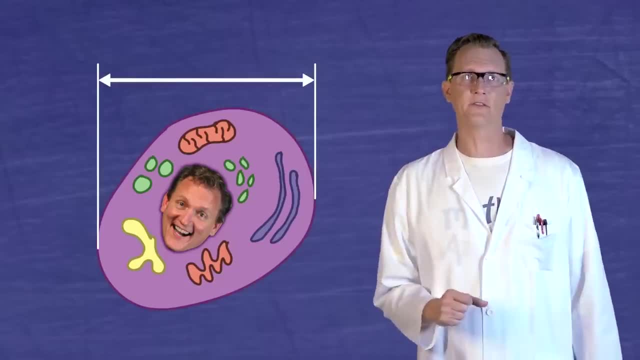 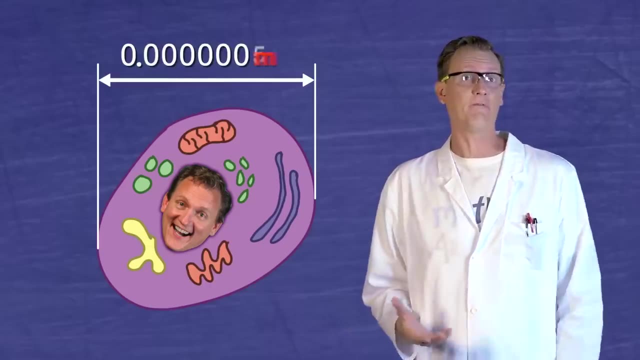 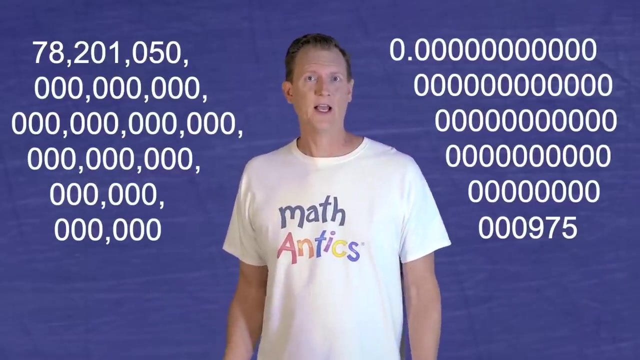 But if you wanted to measure the diameter of one of those cells using meters, you'd get a really small number, Something like 0.00000005 meters. Not only are really big or small numbers, a lot of work to write down because of all the zeros. 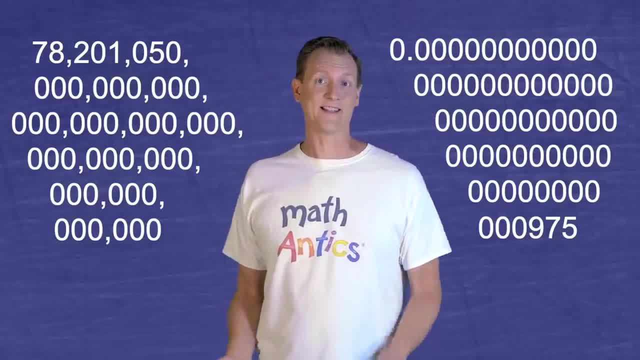 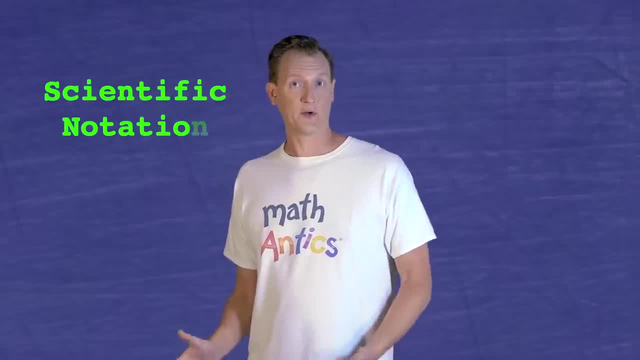 they're hard to quickly evaluate and compare At a glance. it's not easy to tell just how many number places there are in these really big or small numbers, And that's where scientific notation can really help us out, Instead of using a long sequence of decimal digits to represent. 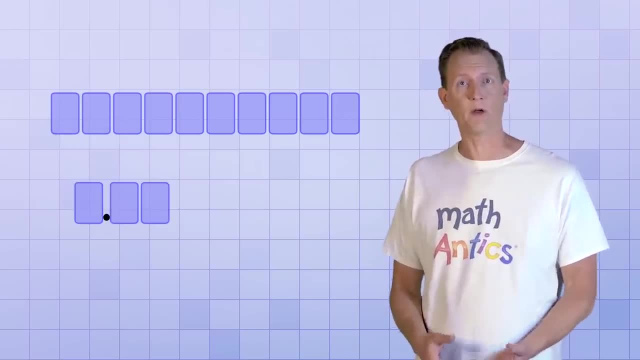 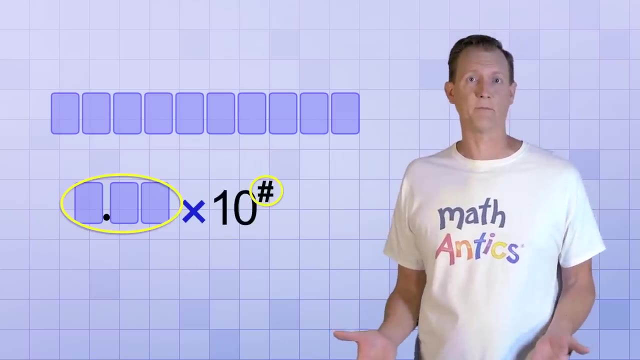 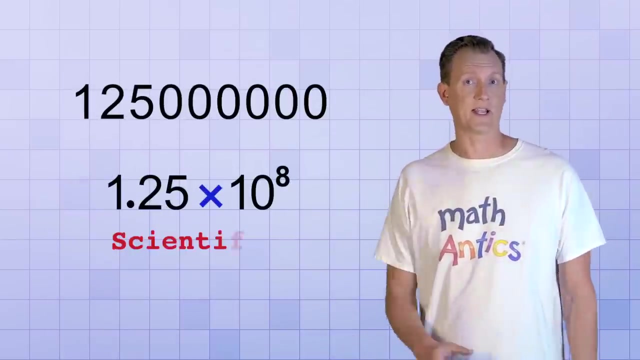 numbers, scientific notation uses a shorter number multiplied by a power of ten, And it's always in that form: Sum number times ten to the sum exponent. Here's an example of a really long number, 125 million, And here's the equivalent number written in scientific notation: 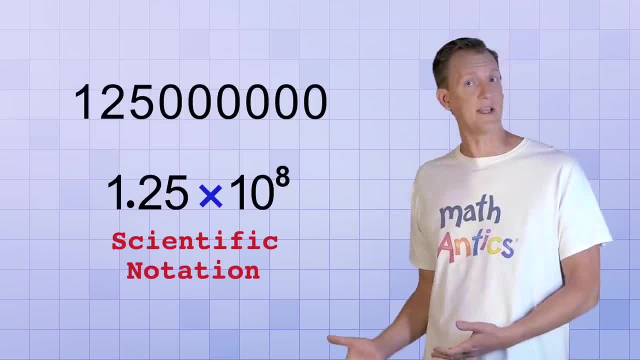 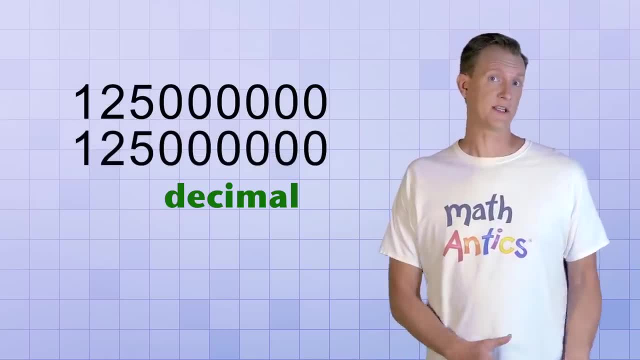 1.25 times ten to the eighth. Want to see how these two numbers are just different ways of writing the same thing. Let's start by making a copy of our big number and messing with its decimal point a bit. Where's the decimal point, you ask? Remember that it's always right here. 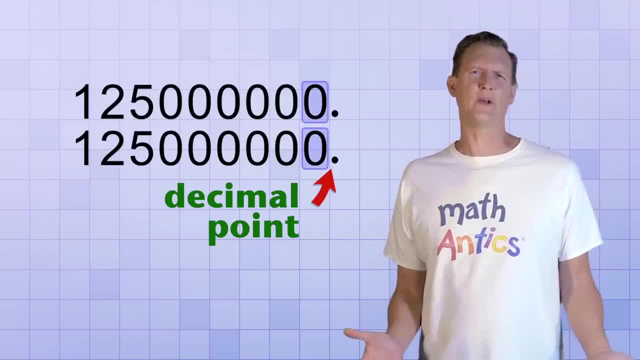 immediately to the right of the ones place. We just don't need to show you the decimal point. Just show it. if there aren't any decimal digits, Ok, see what would happen if we shift the decimal point one place to the left. 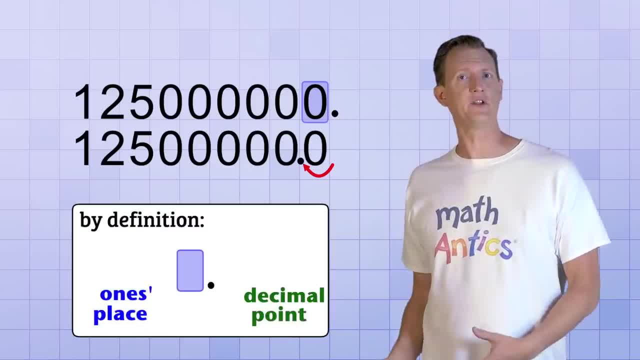 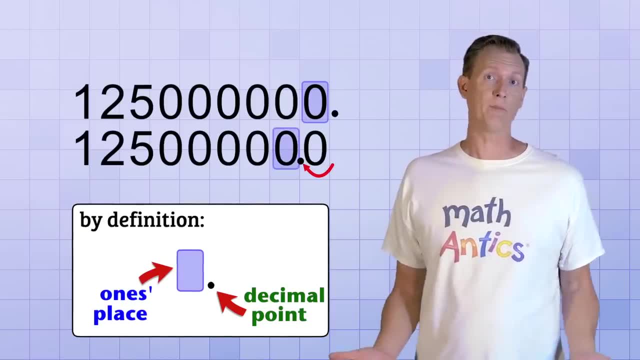 Well, doing that would change the number right. By definition the decimal point always is immediately to the right of the ones place. So shifting the decimal point shifts the ones place and all the other number places too. And if we line up the ones place of our new number with the ones, 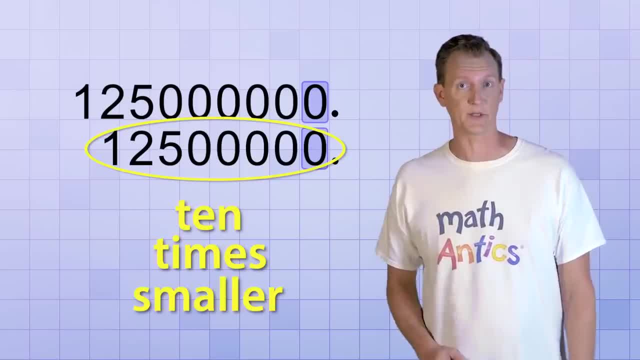 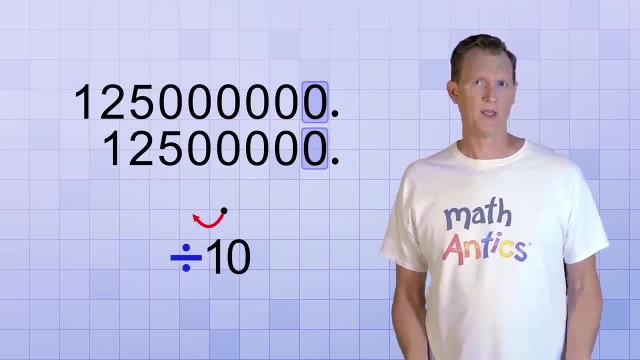 place of the original number. you see that the new number is 10 times smaller. This means shifting point one place to the left is equivalent to dividing a number by 10.. But do we want a number that's 10 times smaller than before? 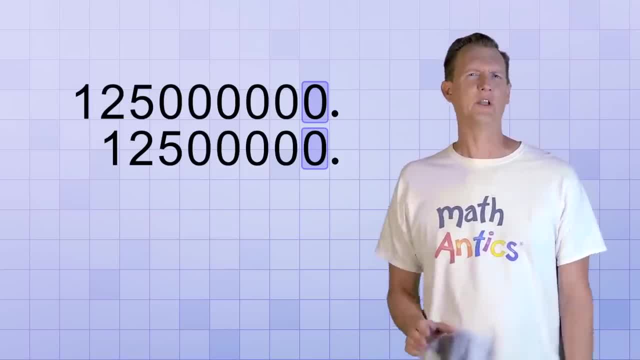 Well, no, We don't want to change the value of the number at all. We just want to write it in a different way, Since shifting the decimal resulted in a number that's 10 times smaller than before. to compensate and keep the value the same, we need to multiply the new number by 10.. 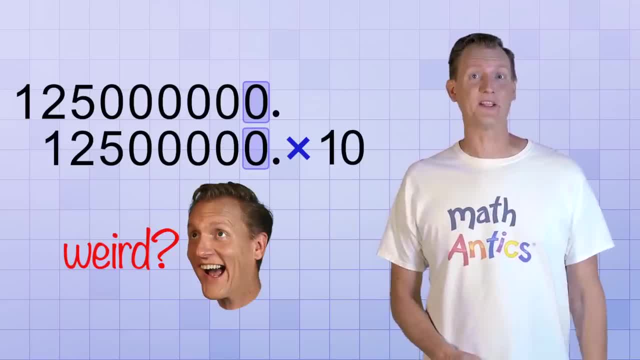 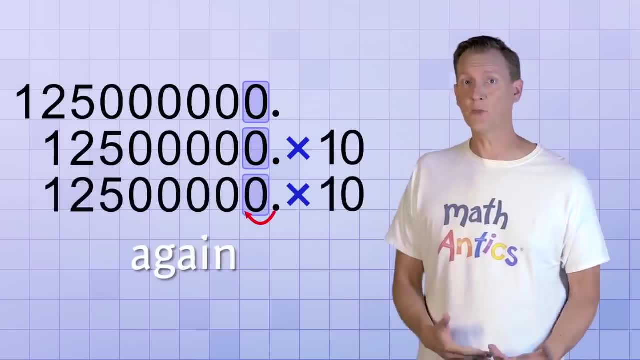 Making the number smaller and then compensating for that might seem like a weird thing to do, but it'll make more sense in a minute. Let's do that process again. Let's make a copy of the new number and shift the decimal point to the left again. 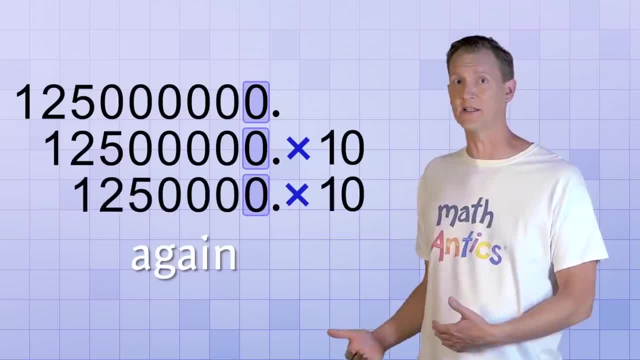 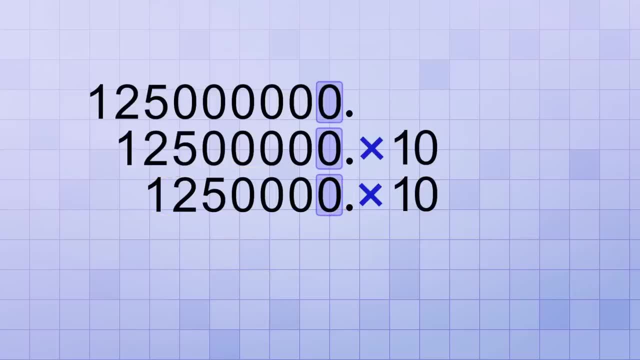 Since that shifts all the number places, we can align the ones places and see that the same thing happened. The new number is 10 times smaller than before, So to keep it the same value as the original number, we need to compensate by making it 10 times bigger. 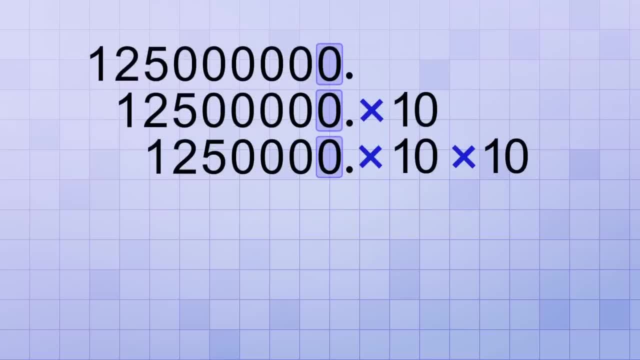 We need to multiply by another 10.. And if we repeat that process again, if we make another copy and shift the decimal point again, we'll see that the number gets 10 times smaller. So we need to compensate by multiplying by another 10.. 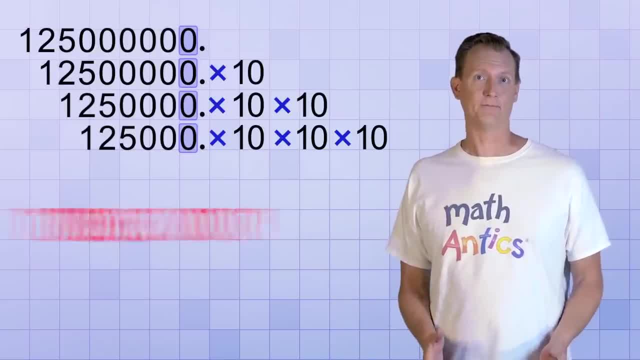 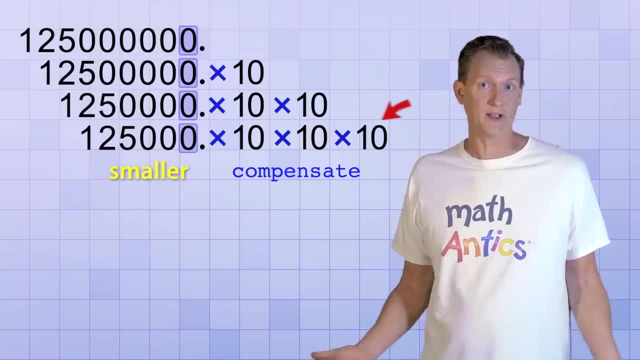 Alright, time out. We seem to have a little problem here. Each time we shift the decimal point to the left, our number gets smaller, but since we have to compensate with a factor of 10 each time, it's making kind of a mess. 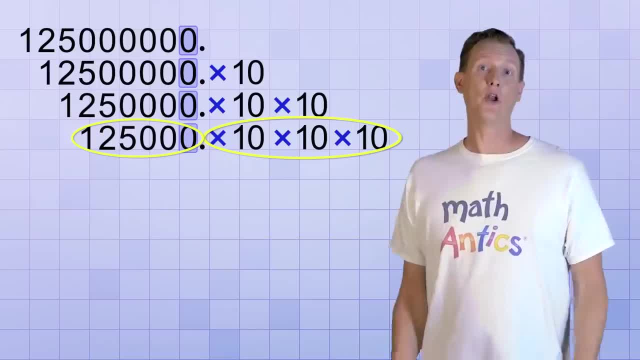 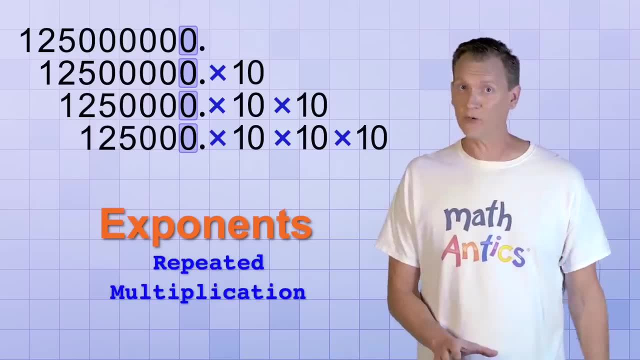 This part's getting shorter, but this part's getting longer. No problem, exponents can fix that. Do you remember that exponents are a way of writing repeated multiplication? If you don't, then be sure to watch our video about them before moving on. 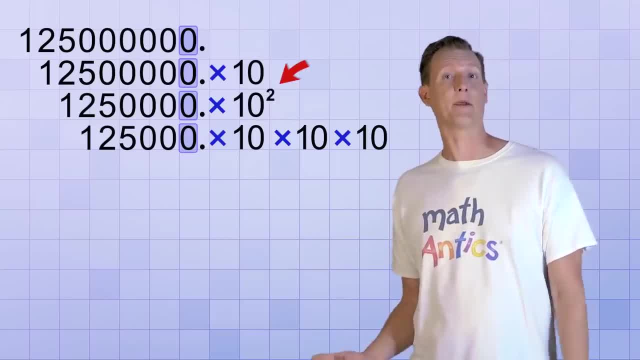 Instead of writing 10 times 10, we can write 10 to the 2nd power, And instead of writing 10 times 10 times 10, we can write 10 to the 3rd power. That's much better. 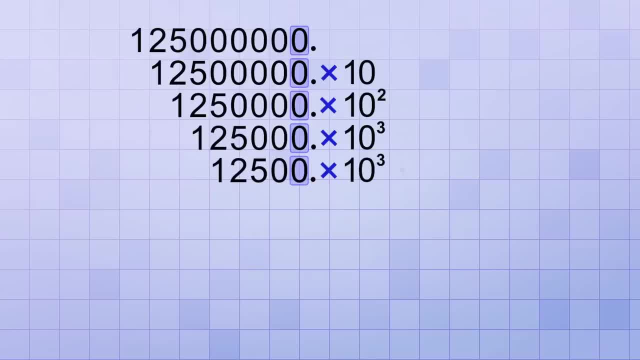 Now we can continue on. We'll shift the decimal point again and multiply by 10 again, But this time, instead of writing another times 10,, we can just increase the exponent by 1,, since there would be a total of 4 10s being multiplied together. 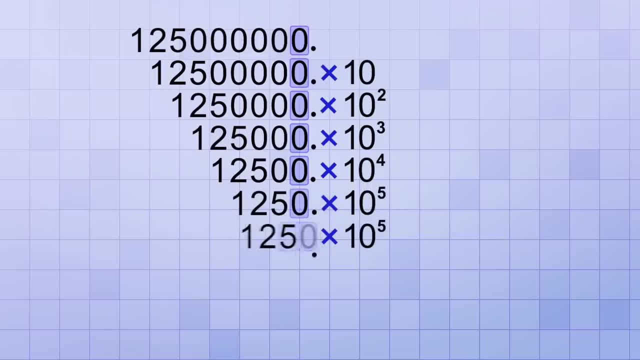 Let's keep going with this process of shifting the decimal point to the left and multiplying by 10 for each number place we shift And we'll stop when there's only one digit remaining to the left of the decimal point. Wow, that's quite a pattern. 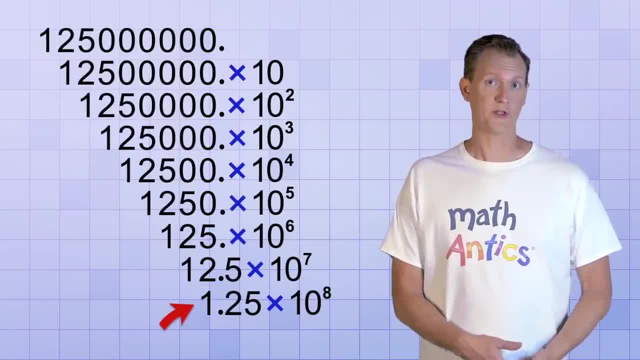 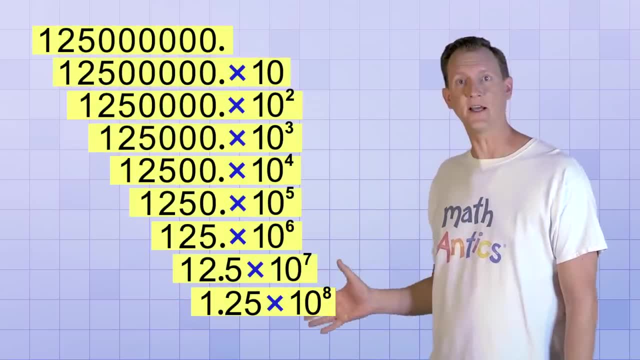 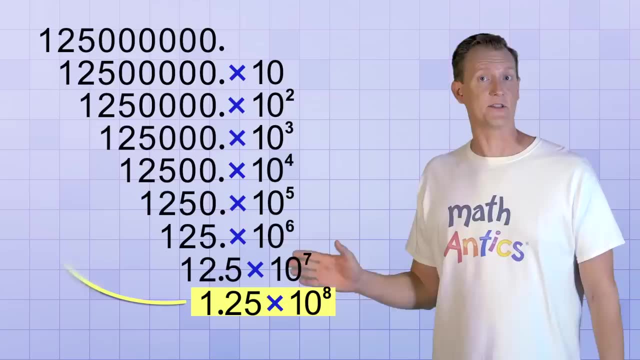 Each time we shifted the decimal, the number got 10 times smaller. So each time we had to multiply it by another 10 to keep the value the same. And because we did that, each one of these lines represents the same value. So, even though it looks a lot different, this last line has the exact same value as the first one. 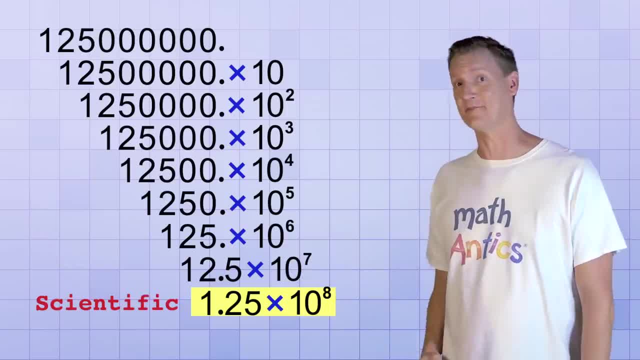 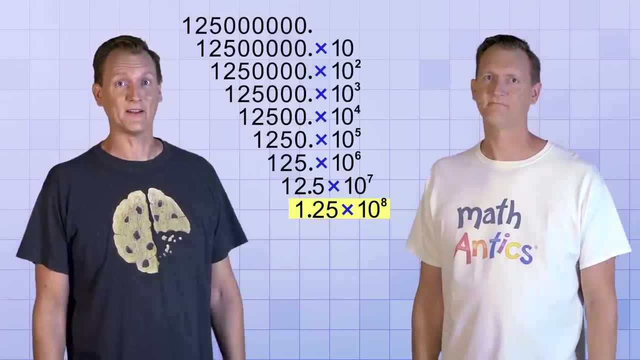 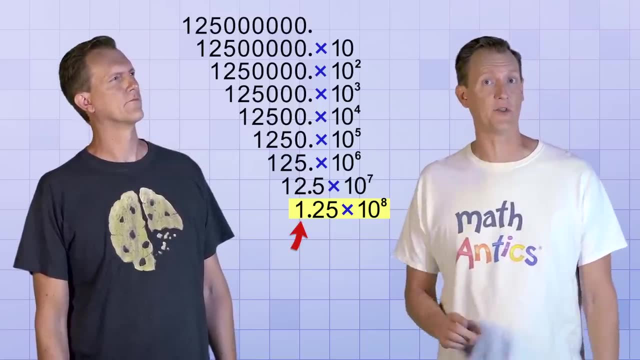 In fact it's just the original number written in scientific notation. But why is it only this last line and not any of the others? I mean, they all look pretty scientific to me. Ah, that's a good question For a number to be in proper scientific notation, it's supposed to have only one digit to the left of the decimal. 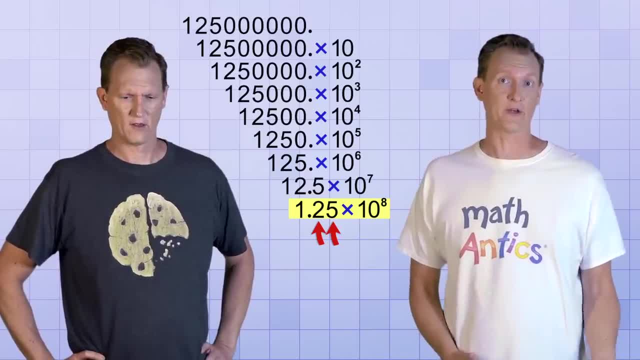 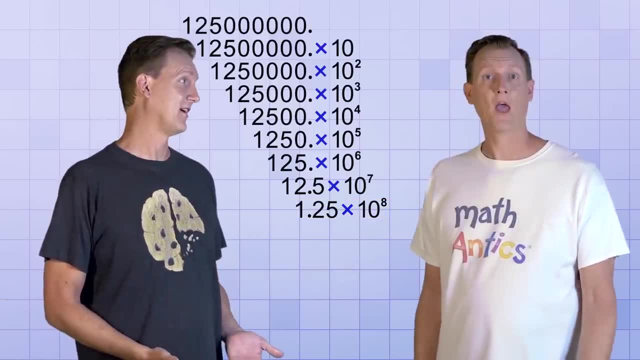 There can be more than one digit to the right of the decimal, depending on the accuracy of the number, but just one digit to the left. But why, I mean? that rule sounds kinda arbitrary. It's not arbitrary at all If there's more than one digit to the left of the decimal point. 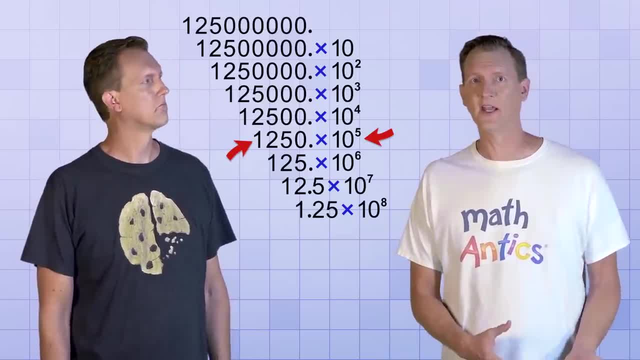 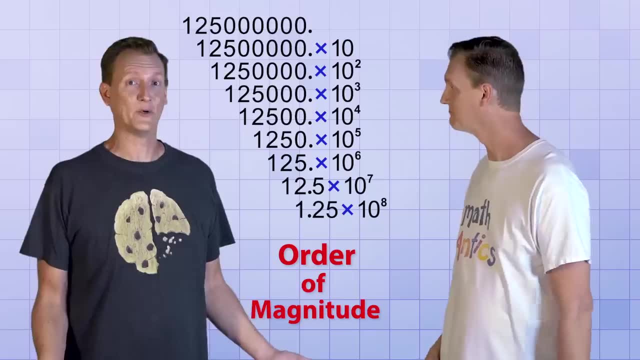 that would mean that we didn't get out all of the factors of 10 that we could have, And factoring out all of the 10s helps us quickly determine a number's order of magnitude. Order of magnitude: What in the world is that? 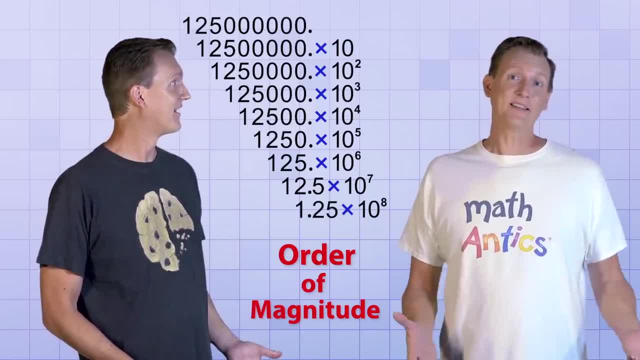 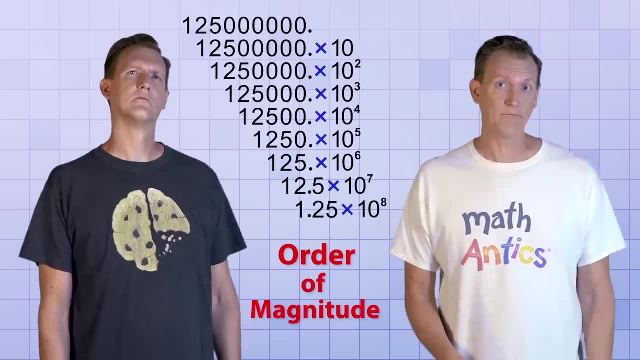 That sounds kinda scary. Order of magnitude is basically just how many 10s you need to multiply to get a certain number, And when a number is in scientific notation, the order of magnitude is just the exponent, because that's telling us how many 10s to multiply together. 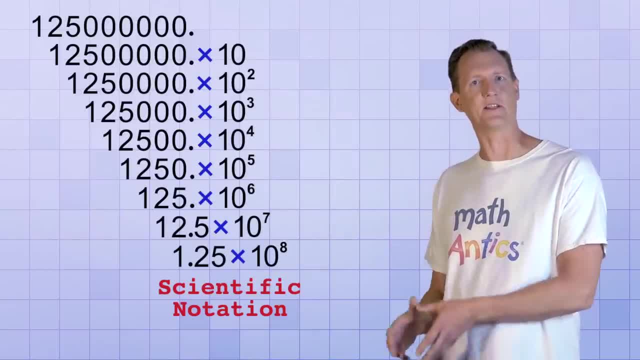 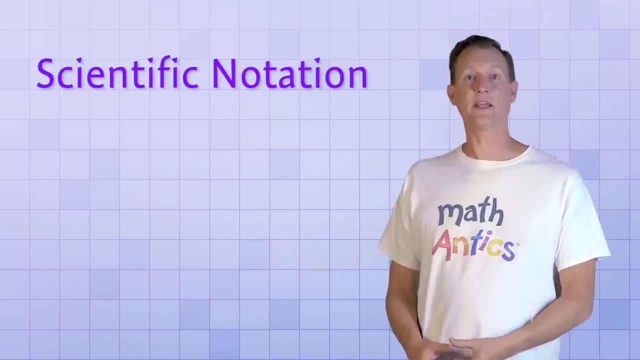 In this example, the scientific notation says that if we take this small decimal and multiply it by 8- 10s, we'll get our original number. So scientific notation is a way of taking a really big number and reducing it down to a value that's less than 10,. 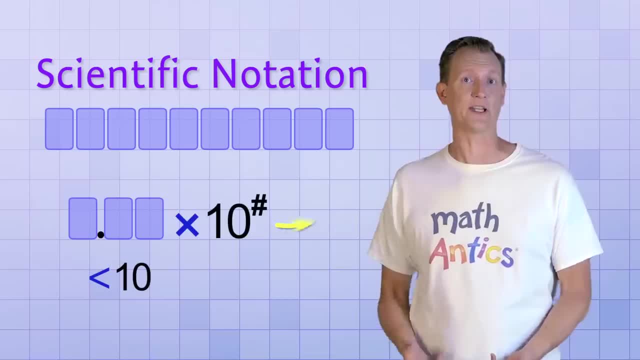 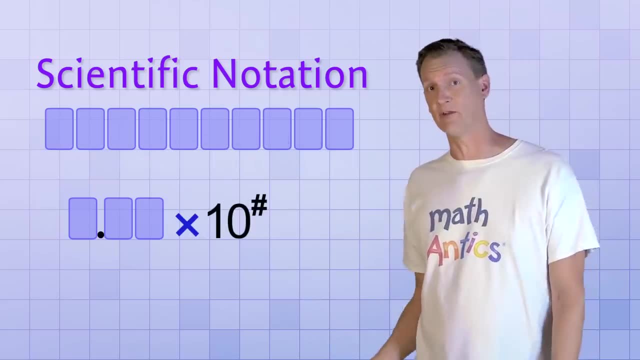 but keeping track of how many 10s we would need to multiply together to get the full number. You can think of it as basically just extracting its order of magnitude and storing it in exponent form. But why would we want to do that? I mean, it seems kinda complicated. 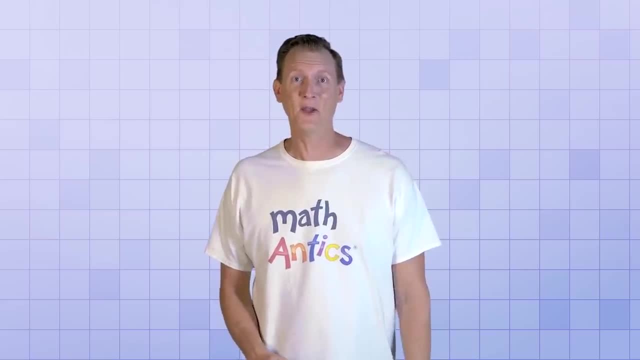 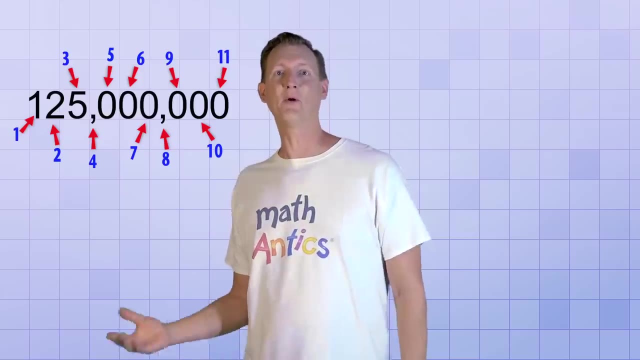 Well, yeah, but did you see how much writing it saved us? When we wrote out 125 million, we had to write 11 characters, including commas. But when we wrote the same number in scientific notation, we only had to write 8 characters. 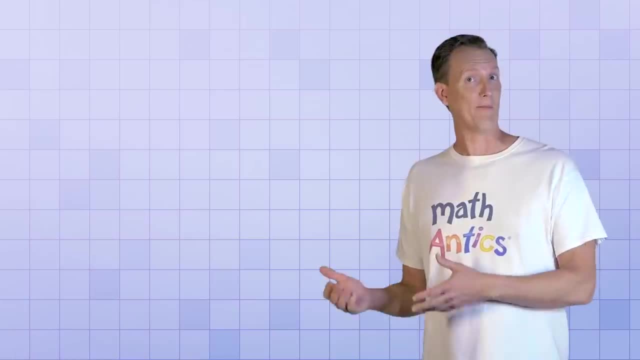 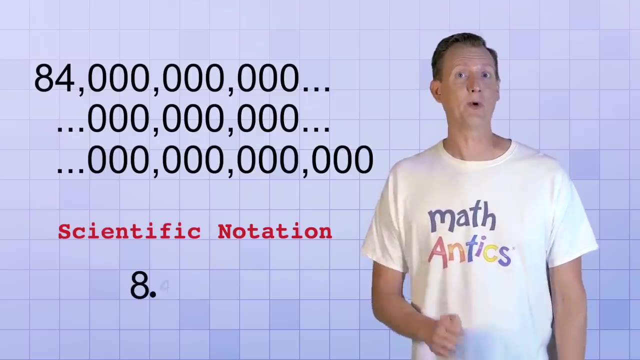 What? Not convinced that it's worth the savings? Well, how about this number? That's a lot of zeros to write, isn't it? But in scientific notation, this number is just a number. This number is just 8.4 times 10 to the 31st power. 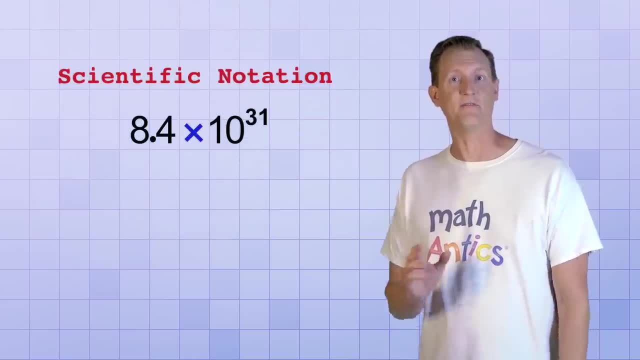 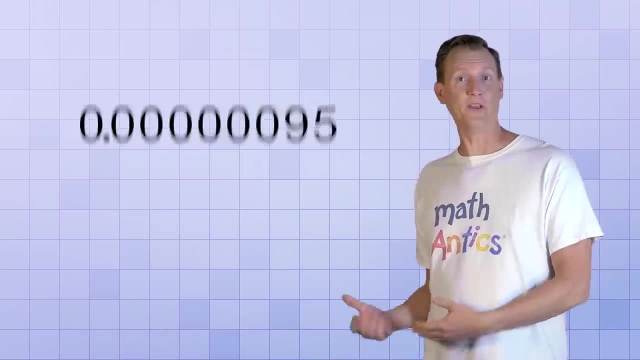 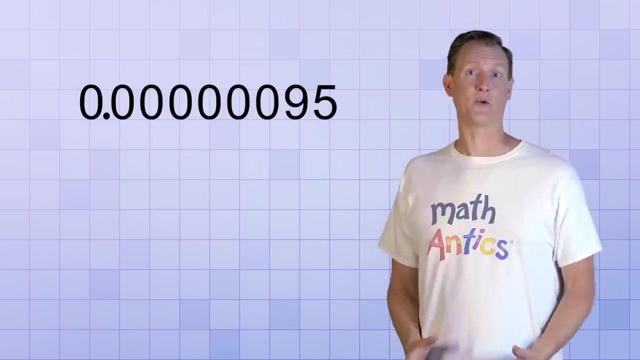 That's much better. So scientific notation is very useful when it comes to writing down really large numbers Or really small ones. For example, this number is really small: 0.000000095. It's much less than 1, but it's not zero. 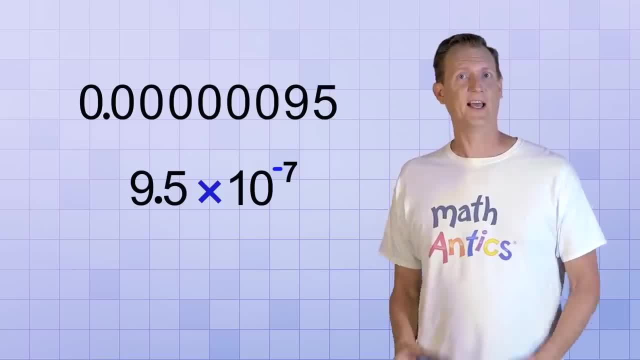 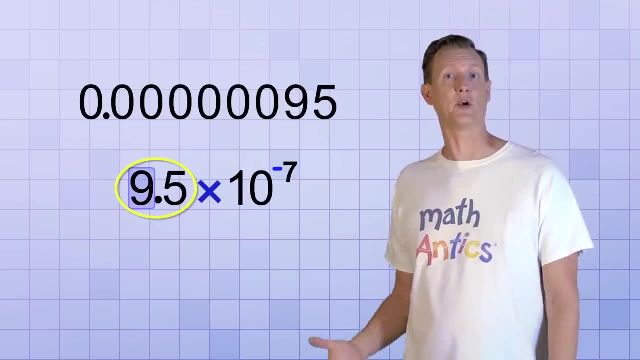 And here's the same number written in scientific notation. Again, it consists of a number that has only 1. One digit to the left of the decimal point, which is being multiplied by 10 to a certain power. But do you notice anything different about the exponent? 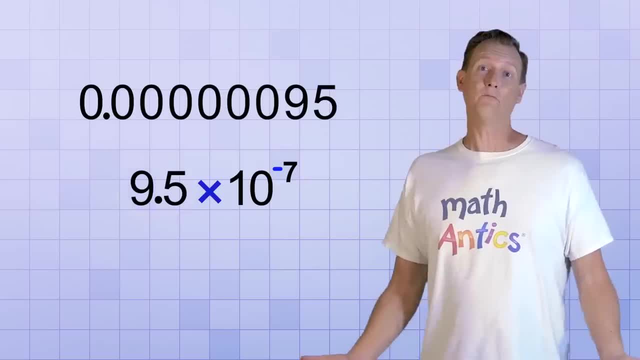 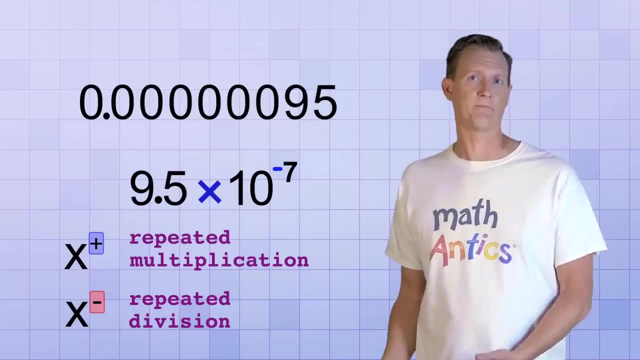 Yep, it's negative. So what does that mean? Well, the short answer is that positive exponents show repeated multiplication, while negative exponents show repeated division. And since this is a negative exponent with 10 as the base, it means to repeatedly divide by 10.. 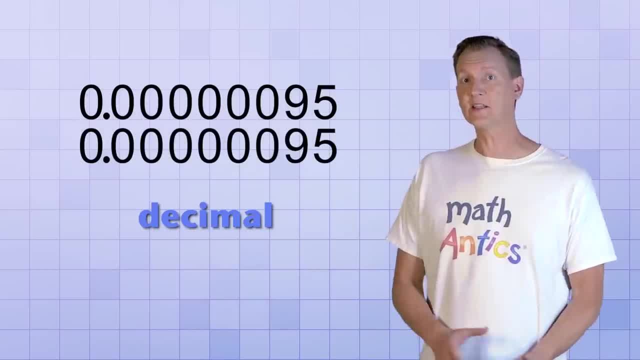 To see how that works, let's copy our original number and do that decimal point shift thingy. And since this is a negative exponent with 10 as the base, it means to repeatedly divide by 10.. To see how that works, let's copy our original number and do that decimal point shift thingy. 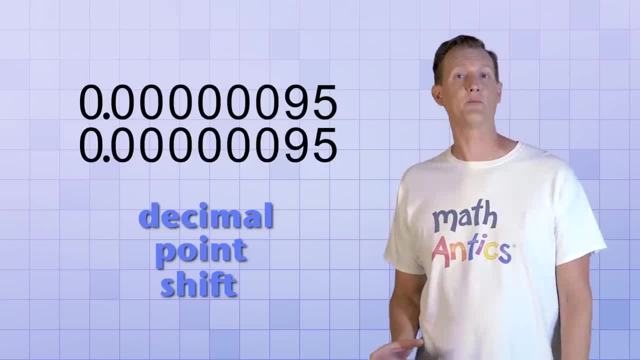 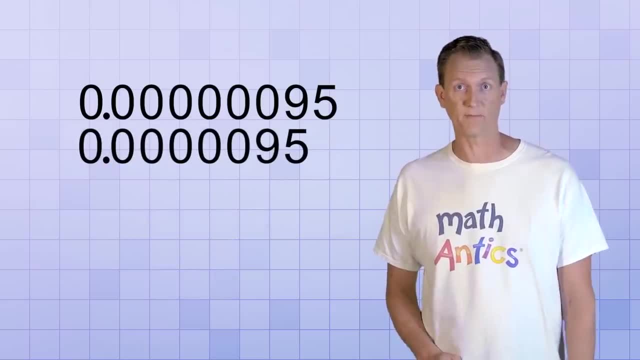 point shift thing again, only this time we're going to shift the decimal point to the right. What happens if we shift it one place to the right? It makes the number 10 times bigger than it was before. There used to be 6 zeros between the decimal point and the 9, but now there's only 5.. 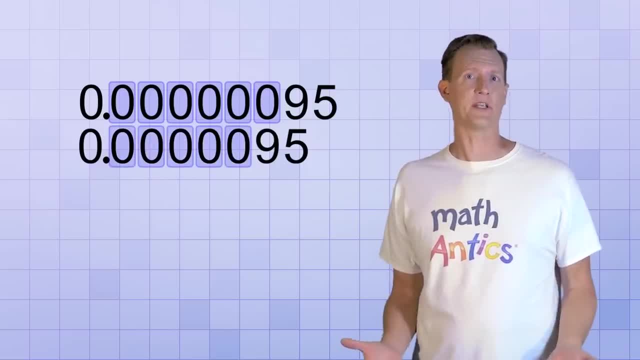 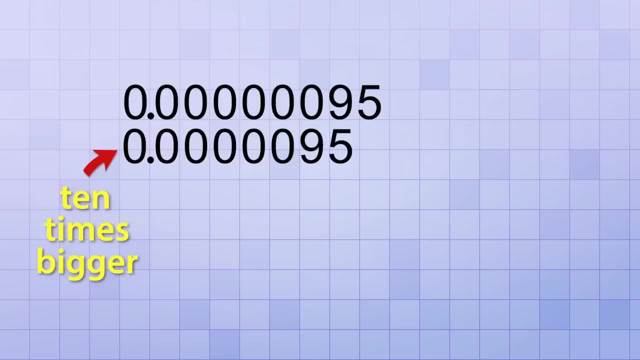 Again, we don't want to change the value. so what can we do to compensate for shifting the decimal point? In this case, since shifting one place to the right made the number 10 times bigger, we need to compensate by dividing the number by 10.. 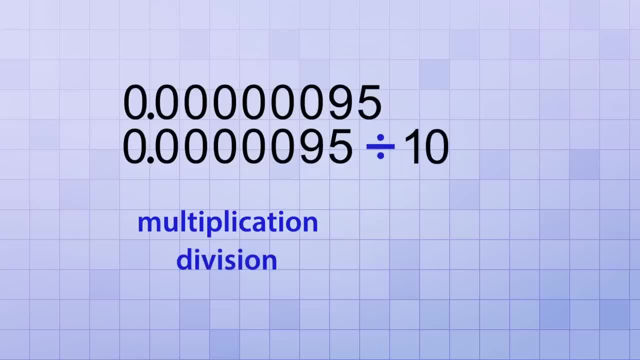 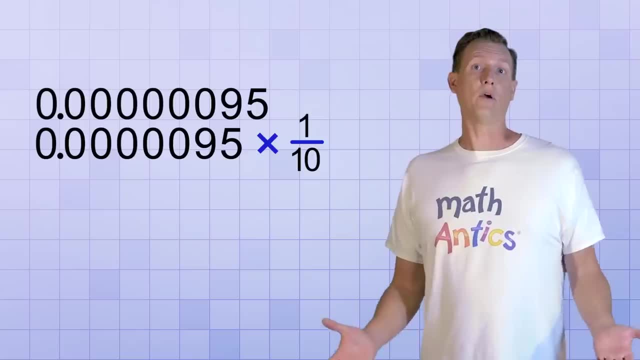 And because the way multiplication and division are related, dividing by 10 is the same as multiplying by 1 over 10, or 1 tenth. so we can just multiply by 1 tenth. Or we can multiply by 10 to the negative 1, because 10 to the negative 1 is just another. 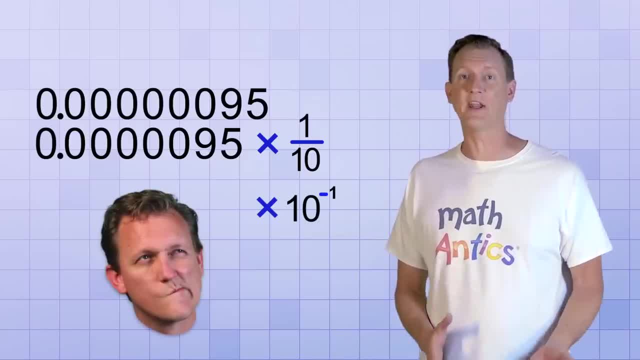 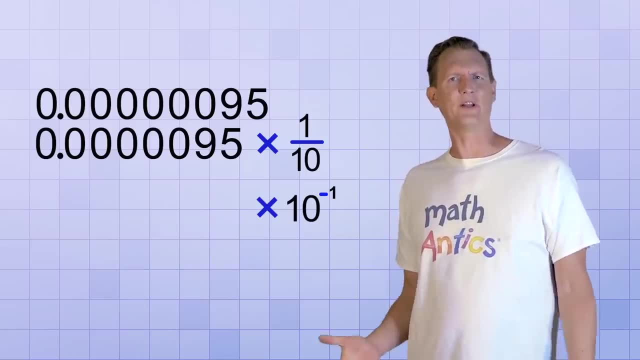 way of writing: 1 tenth. That may seem odd if you haven't learned about negative exponents before, and we explain it in more detail in our video about the laws of exponents. For now, all you really need to know is that multiplying by 10 to the negative 1 is the. 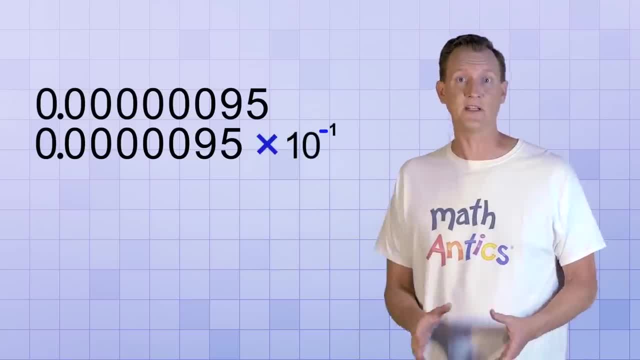 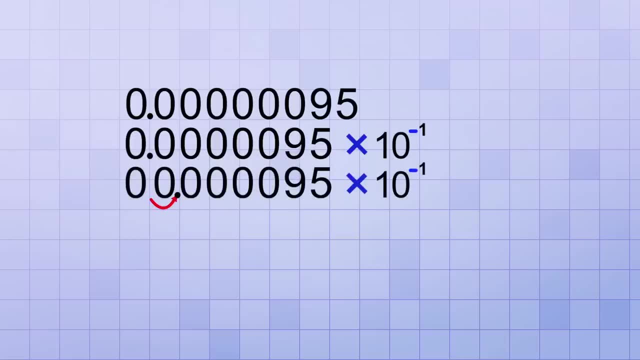 same as dividing by 10 to the negative 1. So it compensates for shifting the decimal point one place to the right, Continuing on. if we shift the decimal point another place to the right, the same thing happens. We make the number 10 times bigger. 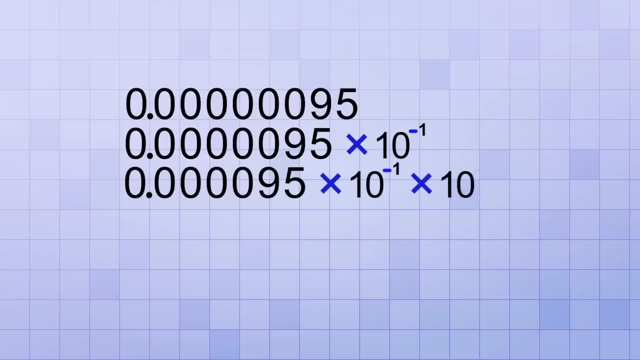 So to keep the value the same, we have to multiply by another factor of 10 to the negative 1.. And if you're wondering whether we can combine these exponents, you're on the right track. 10 to the negative 1 times 10 to the negative 1 combine to become 10 to the negative 2.. 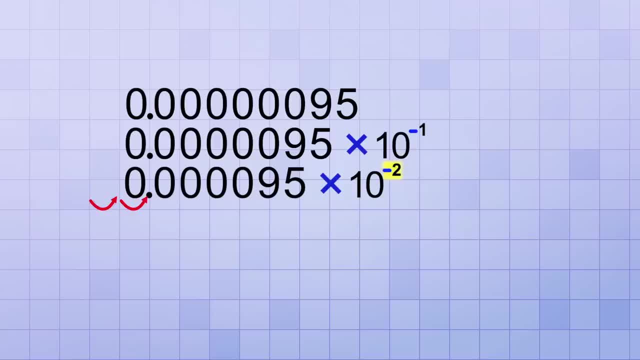 Which makes sense, because we shifted the decimal point one place to the right. So we have 10 to the negative 1 times 10 to the negative 1. And if we shift the decimal point, a total of 2 places to the right. 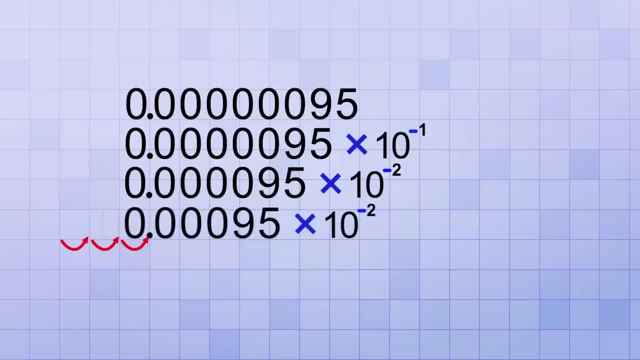 And if we shift the decimal point 3 places to the right, we need to multiply by 10 to the negative 3 to compensate. And if we shift 4 places, then we need 10 to the negative 4 to compensate. Get the idea? 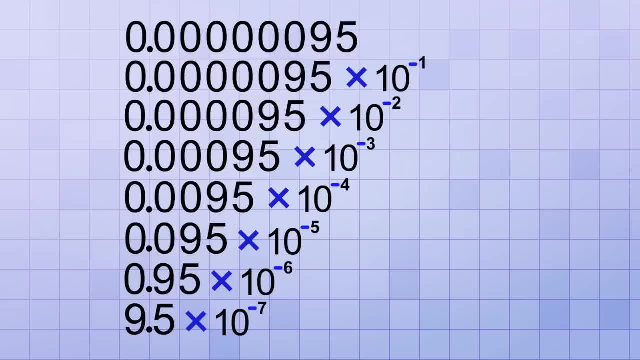 And if we continue doing that until the decimal point is positioned so that there's only one digit to the left of it, that gives us the number in scientific notation, 9.5 times 10, to the negative 7.. And can you figure out what the order of magnitude of this number is? 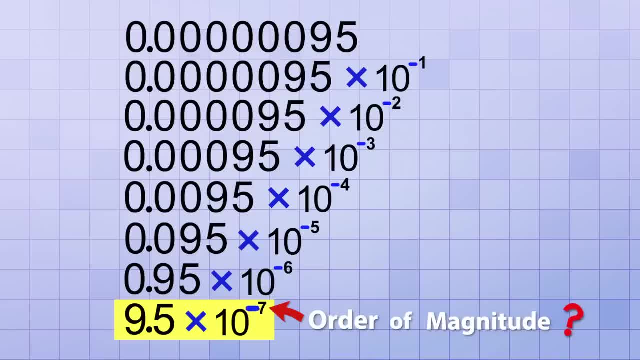 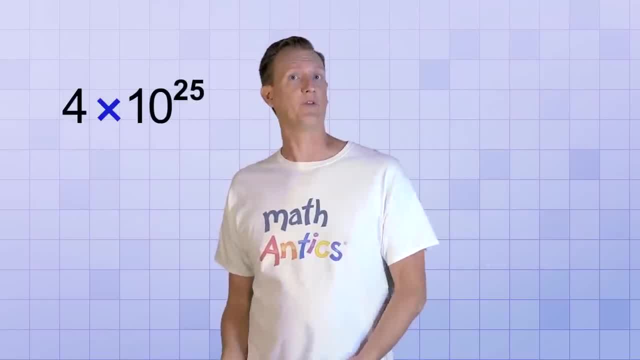 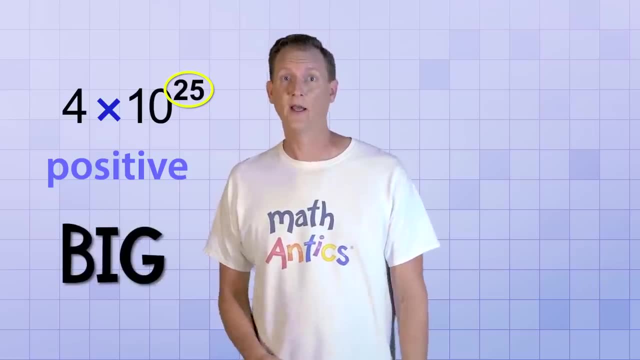 Yep, just like before the exponent tells us It's negative. 7. Being able to quickly identify a number's order of magnitude is pretty handy. For example, if the order of magnitude is a big positive exponent, then you know right away that you're dealing with a really big number. 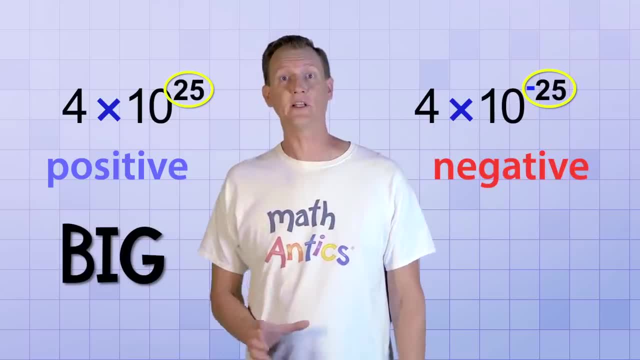 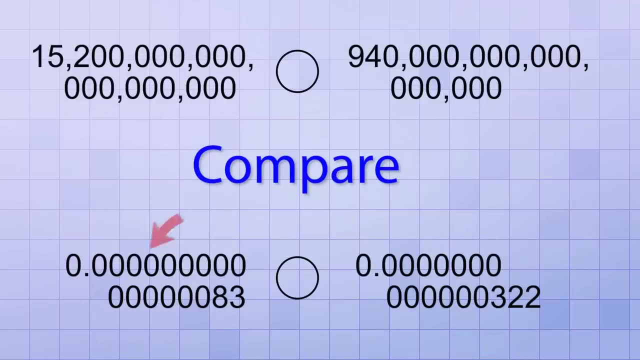 But if it's a big negative exponent, then you know you're dealing with a really small number. And if you're comparing two really big numbers like these two or two really small numbers like these two, it's hard to tell at a glance which is actually bigger or smaller. 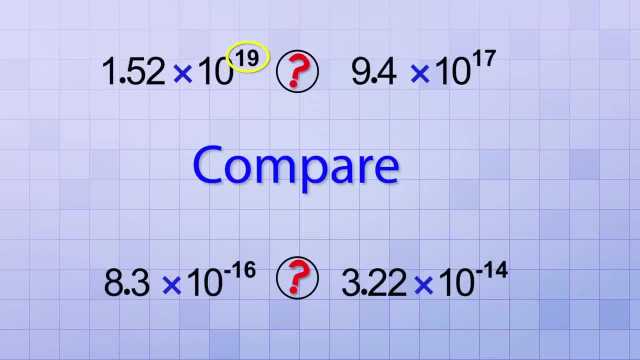 But if you see them in scientific notation, it's easy to see that this number's order of magnitude is bigger than the others, which means that it's bigger, and this number's order of magnitude is less than the others, which means that it's smaller. 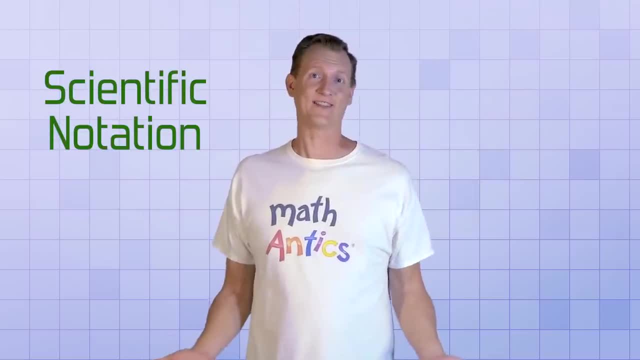 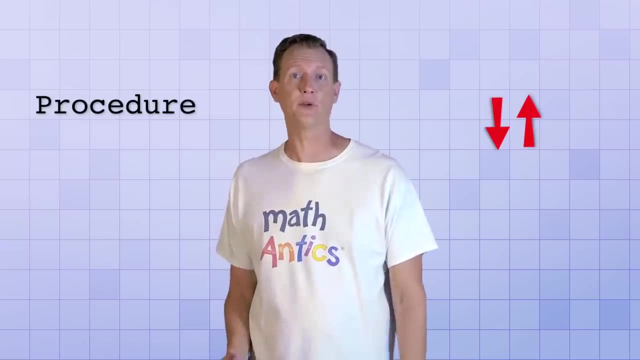 So now that you've seen how scientific notation works and you realize that it's just a shorthand way of writing really big or really small numbers, let's break down the procedure for converting back and forth between numbers written in regular form and scientific notation. 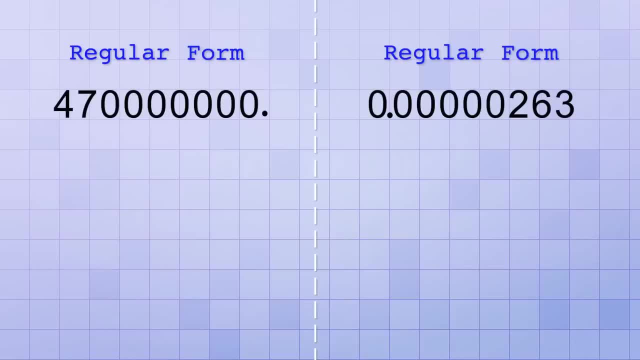 Starting with these two examples in regular form. first, count how many number places you would need to shift the decimal point for there to be only one digit to the left of it. For this number, we would need to shift 8 places and for this number, 6 places. 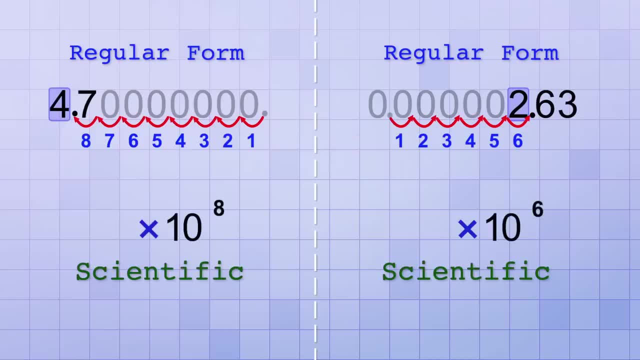 The number of places you need to shift will be the exponent in the scientific notation form, but the sign of that exponent is determined by the direction you shifted. If you shifted to the left because you started with a big number, then the exponent will be positive. 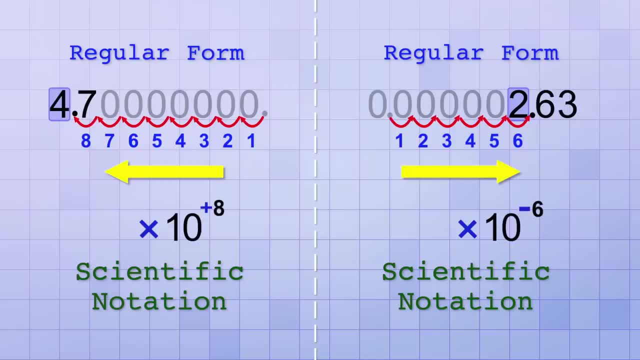 If you shifted to the right because you started with a small number, then the exponent will be negative. So that gives you the times 10 to the something part of the scientific notation. and to get the number that's multiplied by that power of 10, you just take the shifted decimal number. 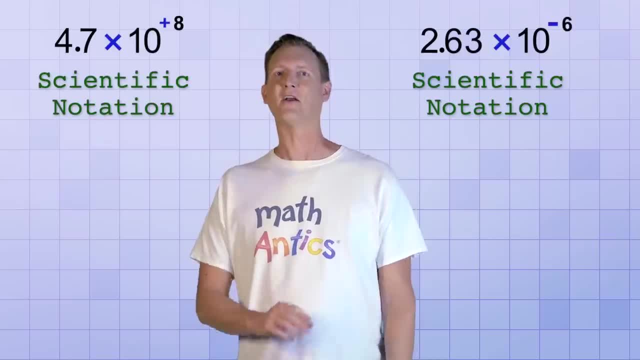 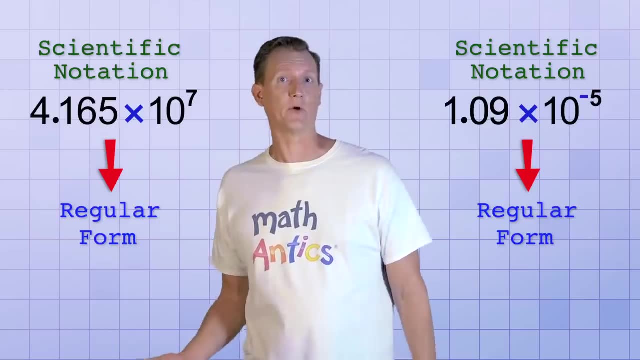 and remove any zeros that don't really need to be shown There. that wasn't too hard, was it? But what if we start out with numbers that are in scientific notation and want to convert them into regular form? Let's do that with these two examples. The first step is to look at the exponent, which is the exponent in the scientific notation. The first step is to look at the exponent, which is the exponent in the scientific notation. The first step is to look at the exponent, which is the exponent in the scientific notation. 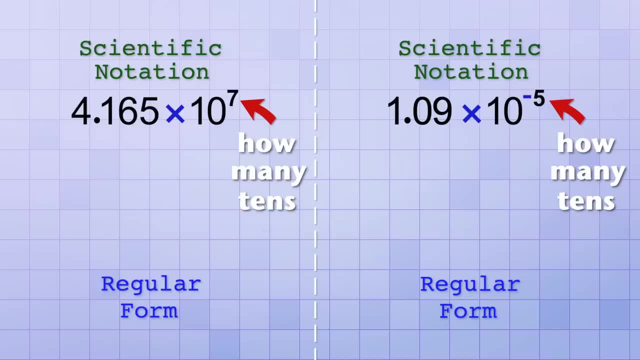 E. 1 is the order of magnitude of the number. It tells you how many tens you need to multiply or divide by to get the number in regular form. If the exponent is positive, it means that you need to multiply by that many tens. In this example, that means we will need to multiply by a total of 7 tens to get the number. 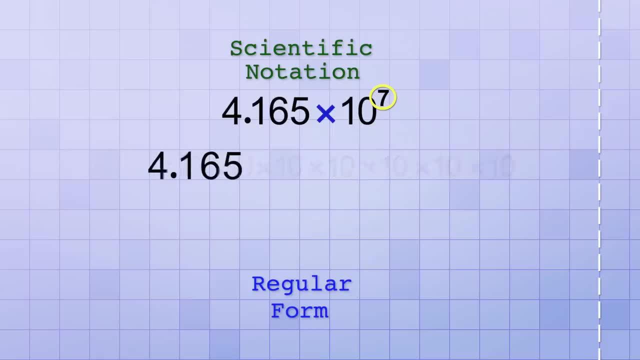 in regular form. That would be a lot of work, but we can also just shift decimal point, that number of places. Which direction do we need to shift it? Well, since we are multiplying by factors of ten, we need to shift it in the direction. 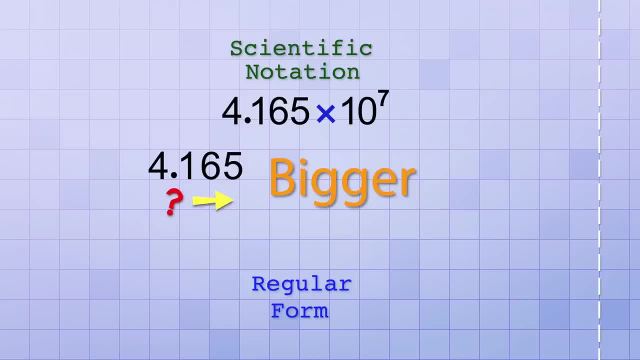 the number bigger That is, we need to shift it to the right. So we'll just shift the decimal point 7 places to the right, But as you can see, there aren't 7 digits after the decimal, So any places that don't. 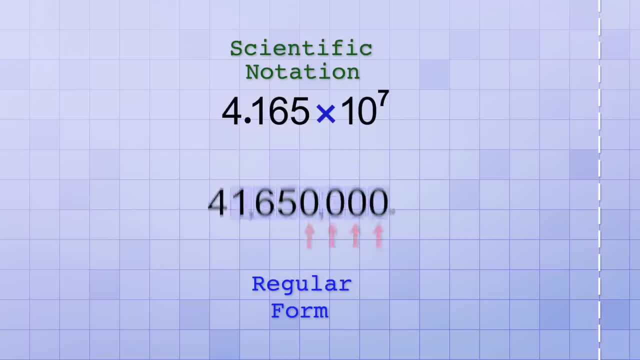 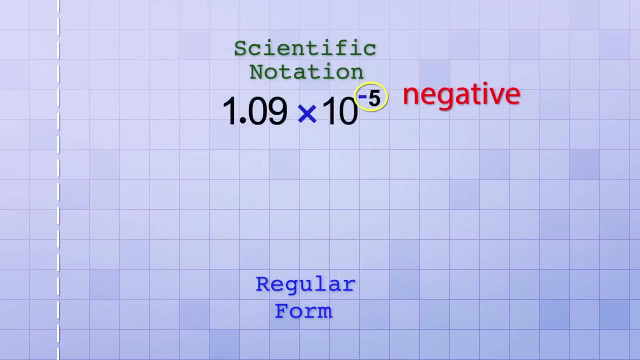 have a digit would just be filled with a zero. There, our number in regular form is 41,650,000.. In the second example, the exponent is negative, which means that we'll need to divide by that number of 10s to get the number in regular form. 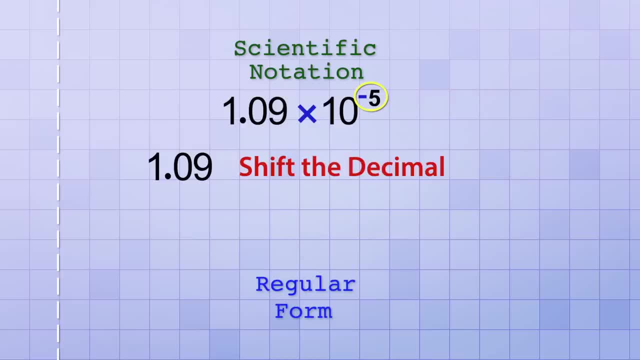 Again, we could just do that division or we can shift the decimal point to save time. Since dividing by factors of 10 make a number smaller, we'll need to shift the decimal point in the direction that results in a smaller number, That is, to the left.